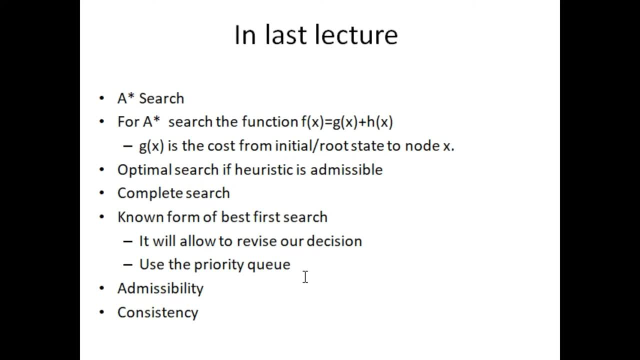 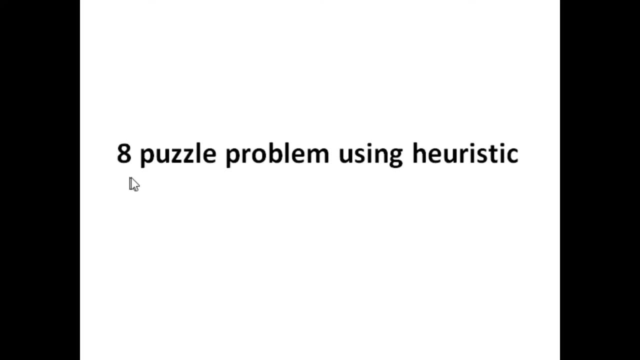 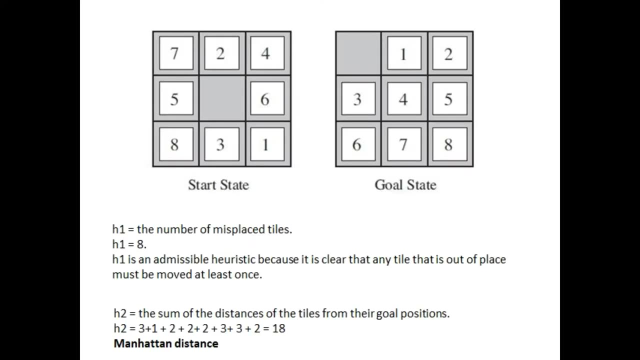 the end of previous lecture we talked about the concept of admissibility as well as the consistency. So in this video we will solve this problem. 8 puzzle problems. So just look at this problem. We talked about this problem in our previous lectures when 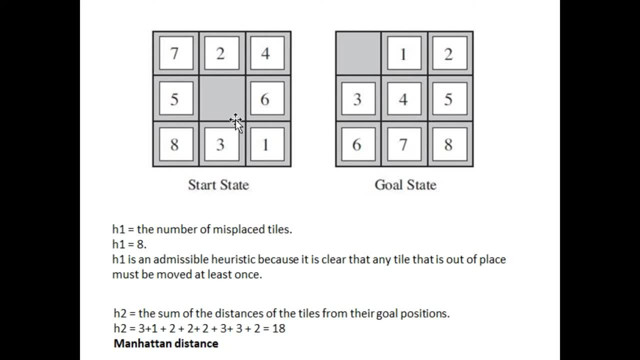 we are covering the problem solving topic, So the initial state is here. There are total 9 boxes and the 8 tiles. each tile have one digit, from 1 to 8, 1,, 2,, 3,, 4,, 5,, 6,, 7,, 8,. 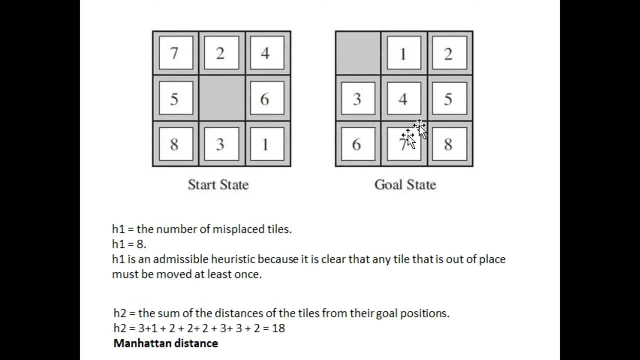 9 up to 8.. In the same way the goal state is here. So the difference between these two states is the arrangement of these tiles. So In our initial state the 1 tile is here. in our goal state the tile 1 is here. In our initial state the tile 2 is here in. 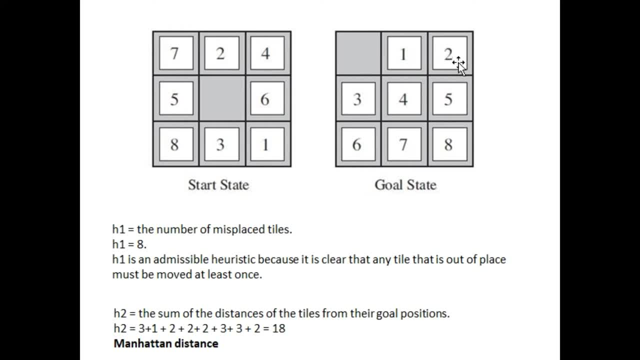 our goal state. the tile 2 is here. we want to move this initial state to goal state and this is our problem and the rule is we can move this empty tile, empty box from this location to right direction in the same way we can move. 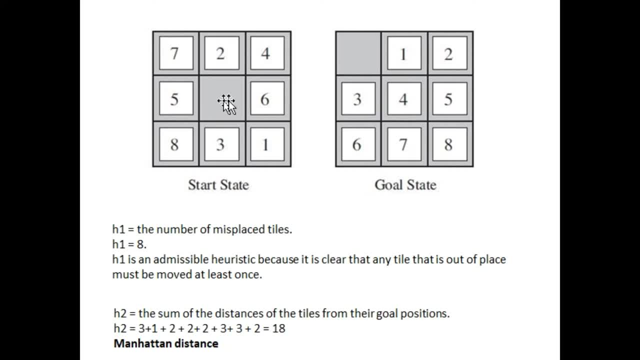 this empty box from this side to left and up and down. so these four are our set of actions. so we cannot move this empty, diagonal, empty, empty box, uh, towards the direct diagonal direction. so so we can move only these four directions. so this is our initial state and this is our. 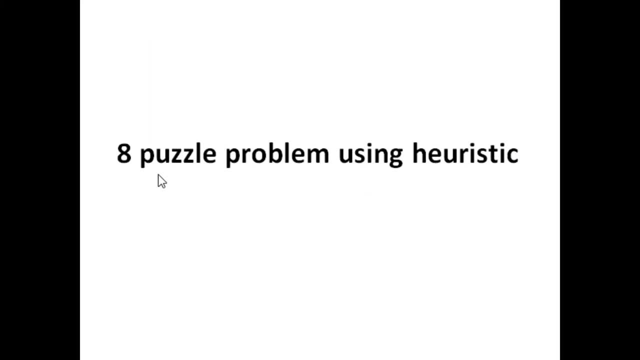 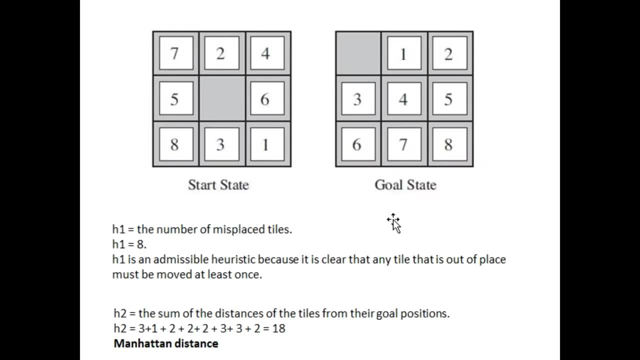 goal state. now, in this lecture, we are going to cover this problem. we are going to solve this problem by using the heuristic. so in our book there are two different ways to calculate the heuristic values. so there are two different ways to calculate the heuristic values. first is the number of misplaced. 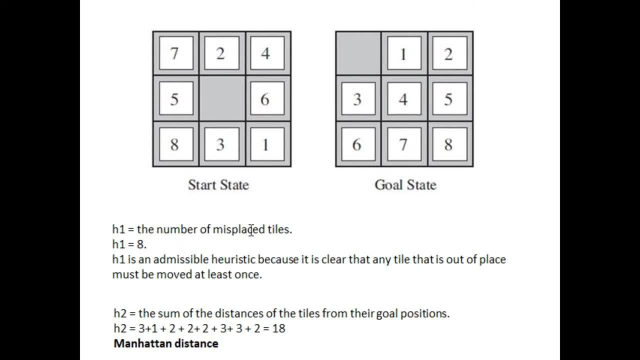 tiles as compared to our goal state. so let's just look at this, that the heuristic value of this math, this initial state, by using this method, the first method to calculate the heuristic value, is 8.. so how can we calculate this? the number of misplaced tile: one is here, but in our goal state the one is here. so one tile one is. 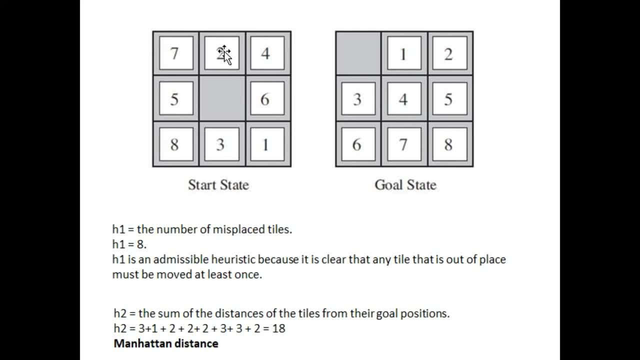 misplaced in the same way. just look at this two we have in the initial state here but in the goal state. it should have been at this point where there is four in the initial state, so the tile two is also misplaced. tile three is also misplaced. just look at this initial state and the goal state location of. 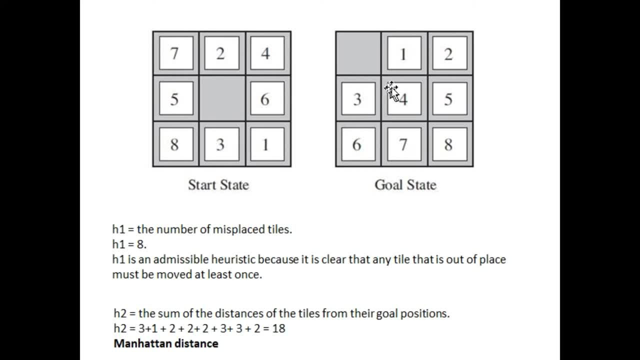 this tile, the tile two and tile three are also misplaced. so, in the same way, tile four we also have misplaced, and the five is also at fault. we also have eight places in all, while the heuristic value of this initial state, which is the start in the first place, 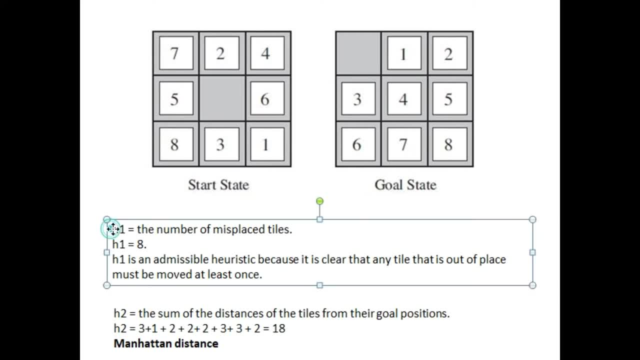 and this start is equal to the start in the second place, based on this method, which is, which is 1 heuristic value is 8, but this is an important point, that the H1 is admissible heuristic. so admissible heuristic, we talked about it. if we want to solve it through A-star search, 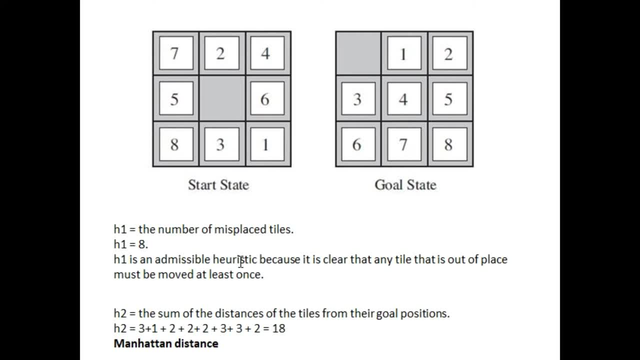 so the first condition for A-star search is that we should have admissible heuristic. so the H1 is admissible heuristic because it is clear that any tile that is out of place must be moved at least once. so at least once it will move. so it means we have to do more movement than that. 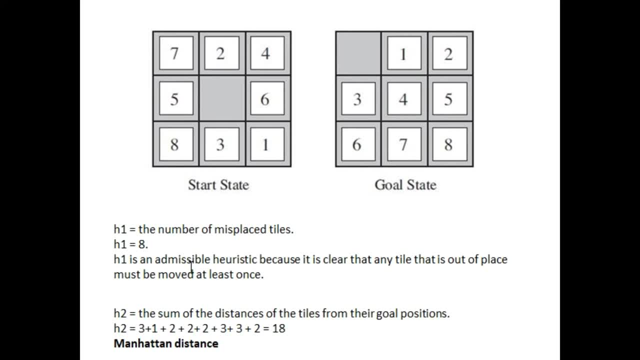 actually. so we don't have overestimated heuristic value, so we will have admissible heuristic. so the second way to calculate the heuristic value, that the H2 is equal to the sum of the distances of the tiles from their goal positions. so and just look at this again, this line, again that the second way to calculate. 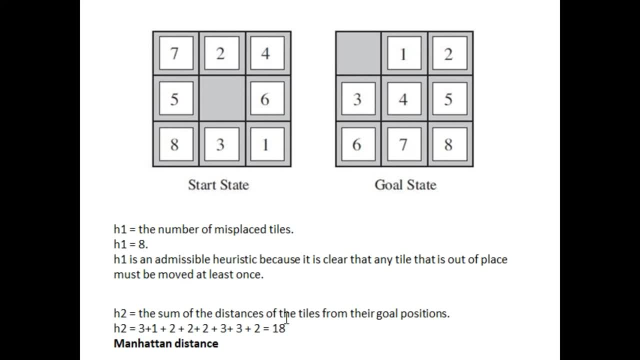 the heuristic value is the sum of the distances of the tiles from their goal positions. so how can we calculate the distance? we will use the mad hat and distance. just look at the heuristic value, that H2. I mean this initial state, for this start state, the heuristic. 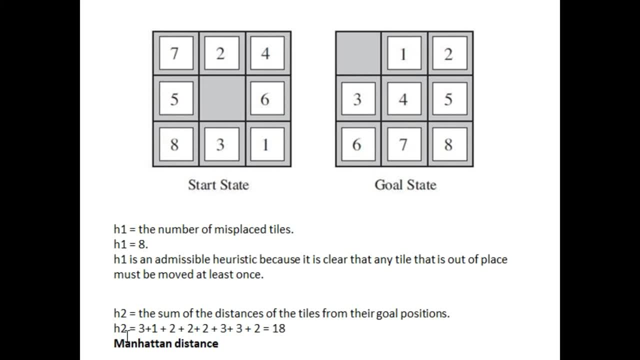 is 18 by using this method. So I will now see how 3 came, how 1 came, how 2 came In the same way, how all these values come By using the Manhattan distance. so let's explain this a little. So just look at this value 3.. So this is for tile 1.. So just look at. 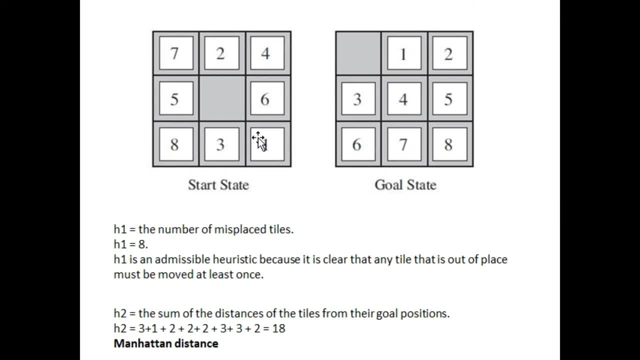 this In our initial state. 1 is here, But in our goal state, so the tile is here. So how will we take this? How will we calculate its distance So we can move from this state to this state? Then we will move towards this state. In the same way we will move towards. 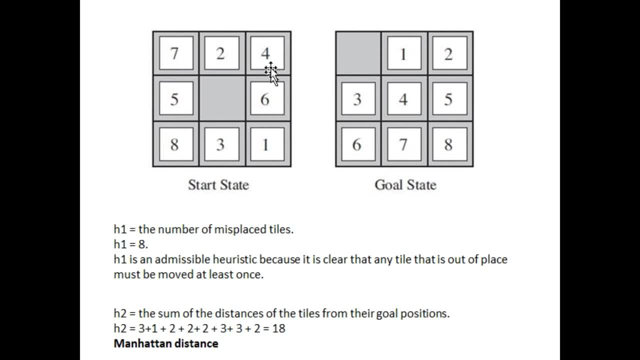 this state. So we have 3. What will it do? It will cover, So that's why we have its value 3. In the same way for 2.. So just look at this: 2. So how did we get 2?? Because the distance. 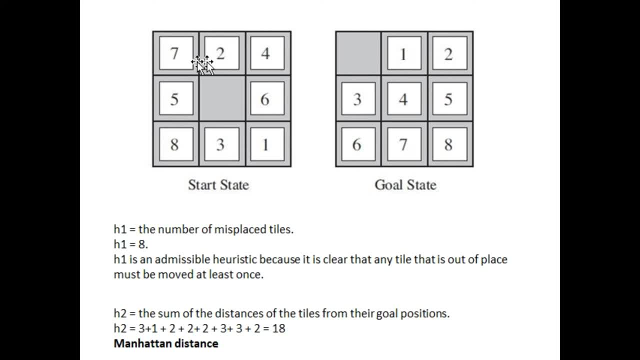 of 2 is. if we compare it with our actual tile, with the goal, then it is 1.. So the value for 2 is 1.. In the same way, just guess and tell me that, this 2 that I have highlighted- 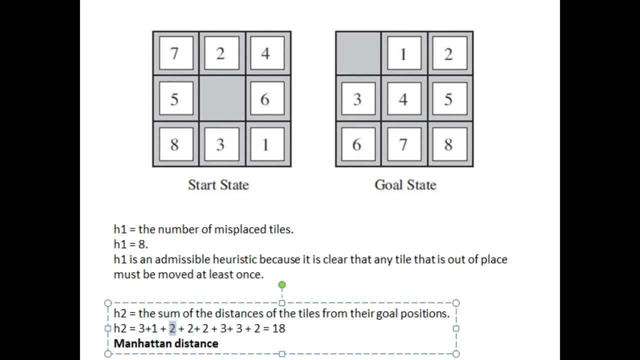 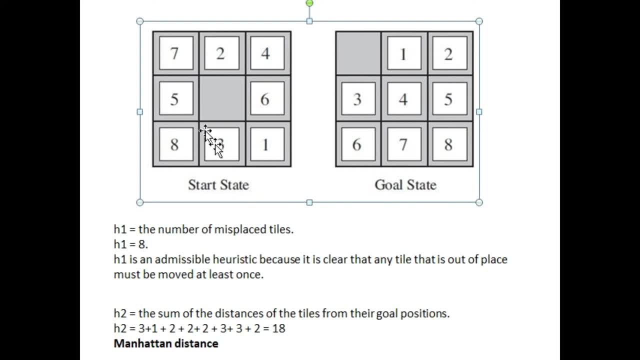 tile 2.. See, just look at this point. We cannot calculate its distance this way, by Amen 3. We cannot calculate its distance by using the diagonal direction. So we can move this tile from this location to at this location, In the same way we will move this tile from. 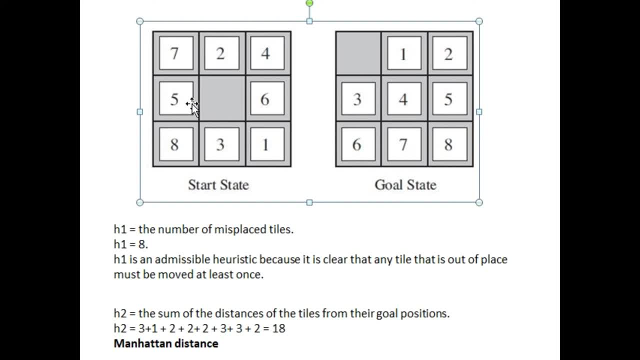 this location to that location. So the total difference we have is 2.. So here I have written: 2.. In the same way for tile 8, actual distance, actual location for this tile is 1.. So I can put 1.. So then the total distance is 1.. So the total distance here for tile 8 is 2.. Okay, So the total value of tile 8, wise as I gave, Or that for tile 8, if we thought. 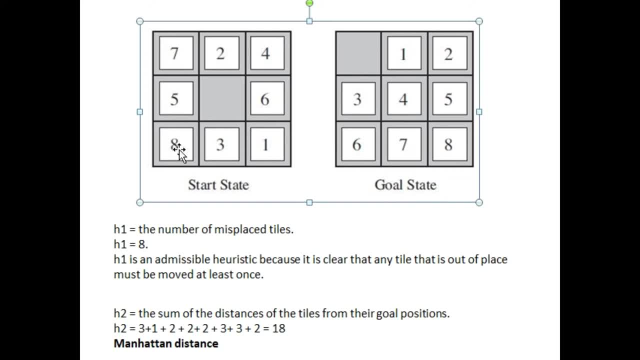 the total difference of tile 8 is one, so that the total air diseases are not satisfied in. the tile is here, but in our initial state the tile is here. we can move this tile at this direction, at this location, in the same way we can move this tile from this location to this location. so 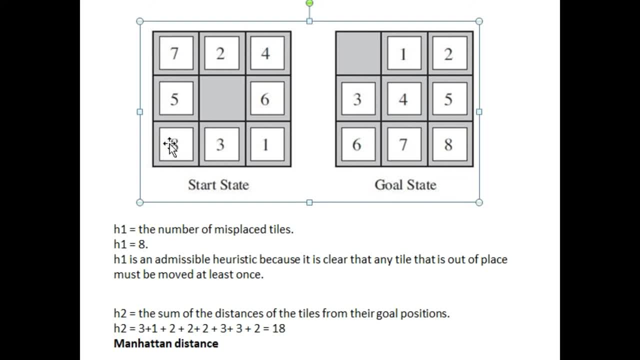 the distance between the for this tile 8 is 2, so just two locations. just add up all of these values. so this is the heuristic value for our initial state for this state. so just look at this value. this is the heuristic value for our initial state to reach goal state. 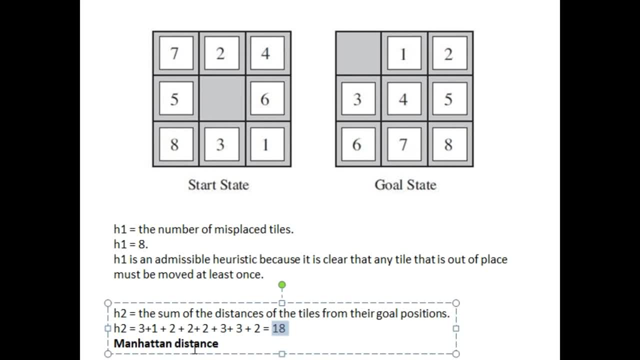 How can we calculate? we calculate by int coin distance. under this slide we covered the two different methodology to calculate heuristic values, and the first one is number of misplaced tiles, and in the sa� i balanced them and the small part of this list with length way. the second, second method to calculate the heuristic value is the sum of distances of the. 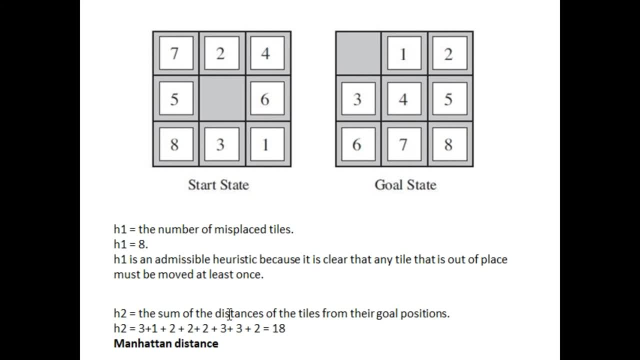 tiles from their goal positions. so we can calculate these distances by using the manhattan distance. so now i will solve this problem, uh, by using the heuristic values. so, because this is this is a very lengthy problem, that if we want to solve this problem, so just i. 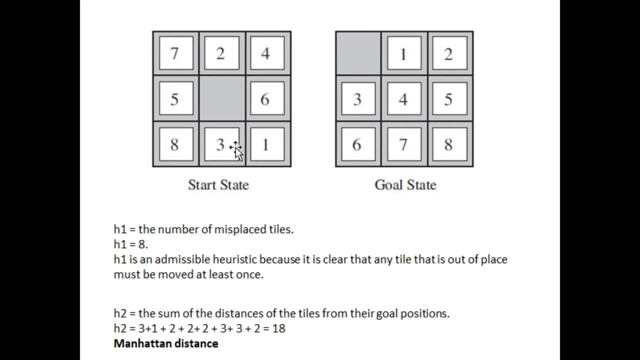 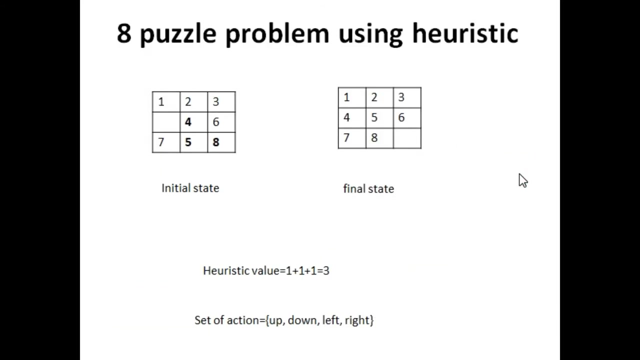 will change the initial state and the goal state in the same way. i will pick that, uh, that initial state and the goal state. this message is so just look at this problem- that i have changed the initial state as well as the goal state. so this is our initial state and one, two, three, four, six, seven, five, eight. so just look at this arrangement. 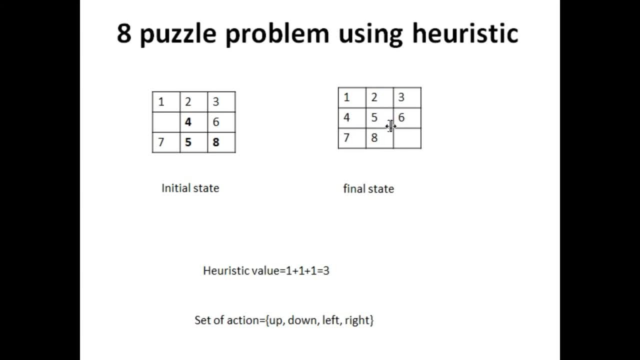 the same way. the final state is one, two, three, four, five, uh, six, seven, eight. so this is our final state. so, uh, initial state, final state. what is the set of action? we can move this empty box in upward direction in the same way down left and right. so other kcb, if any problem have. initial. 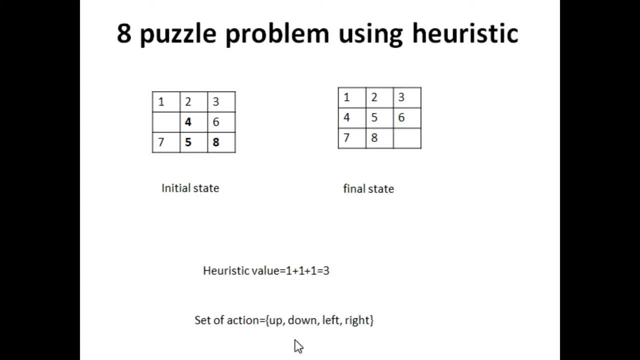 state, final state and set of action. we can say that, uh, the problem, the the problem is is a well defined problem. so just look at the heuristic value. so the four, uh, the in our initial state four is here, but in our goal state four is here. so in the same way, in our uh five, if in our initial state the five 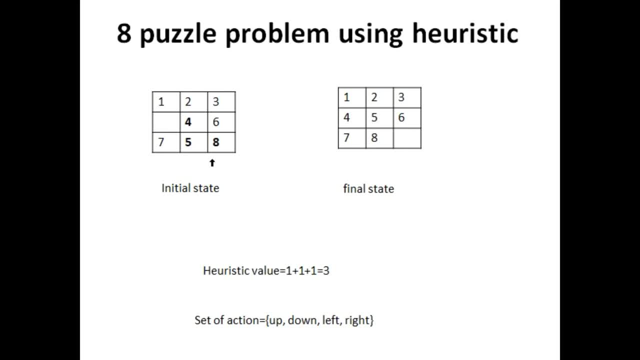 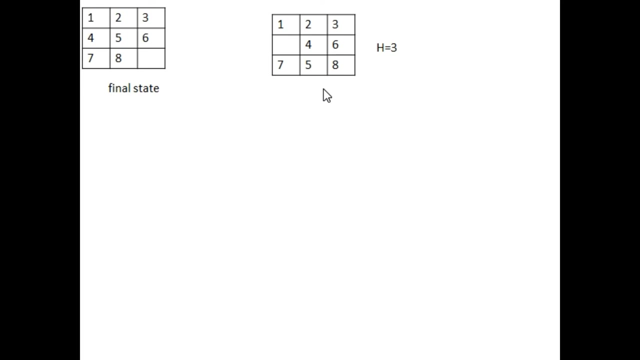 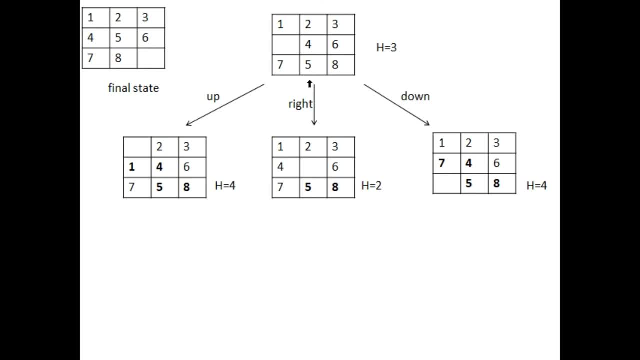 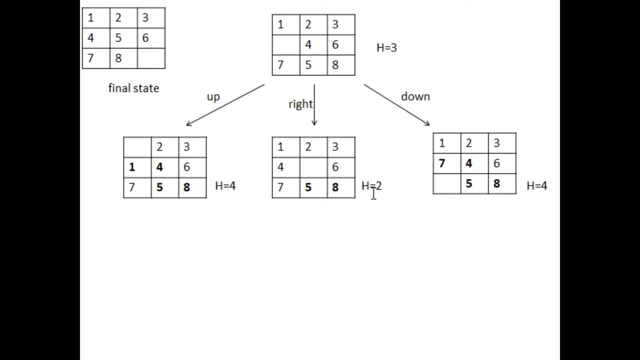 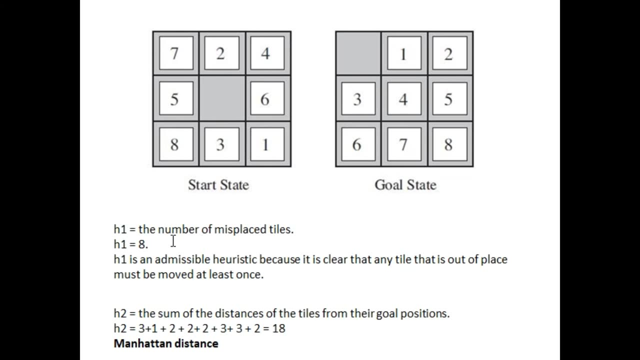 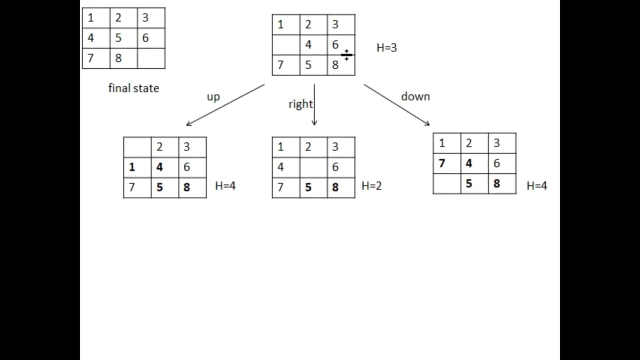 the using both methods, as we discussed in our previous slide. by using this method, the number of misplaced tiles and the second method is the sum of distances of the tiles from their goal position. so in the same way you can calculate this. the heuristic value for this state, so 7 is also not in our actual location. 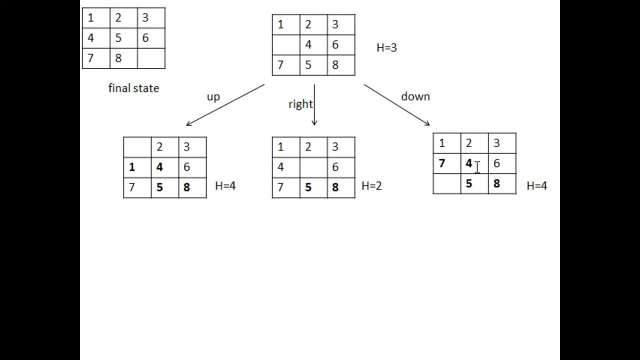 in the same way: 4, 5 and 8. so the heuristic value for this, for this state, is 4. so the heuristic value for this state: 4, 2 and 4. so in which direction will I go? so I will pick this node because the heuristic value is 2, so this state. 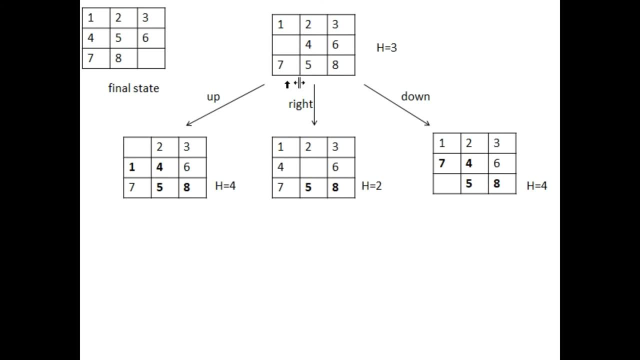 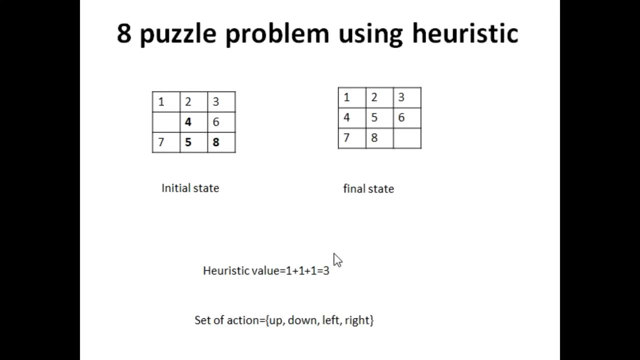 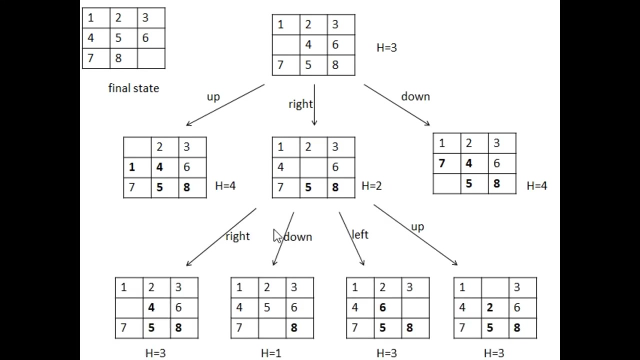 claims that if I move from this initial state to that state, so in my next two steps, what I will obtain is the goal. I will apply these, all of these set of actions, up down left and right at this state. so just look at this slide. I apply it. all of these actions right down left. 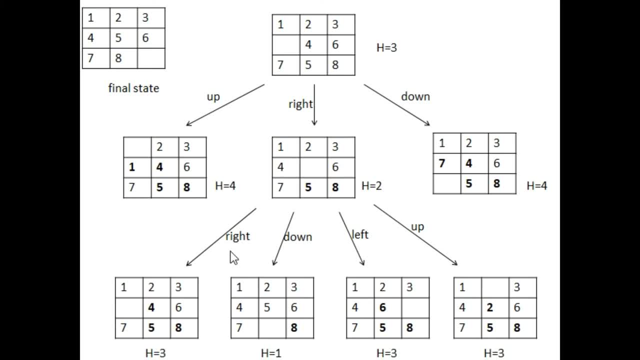 and up on this state. so when up when I apply, the right and left has two steps in it, so big and small with respect to three steps and then to the last. then we have again the upper half, which is 2 together on the Mos ils and E ball and then E rt equal. 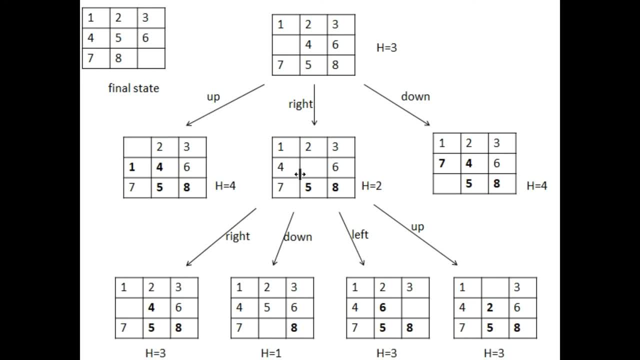 action on this state. so just look at this, the box move at this direction. so then i will calculate the heuristic value again. so the heuristic value for this node is three. in the same way when i apply the down direction action. so if five go up or five empty box, so at this, uh, for this state, the 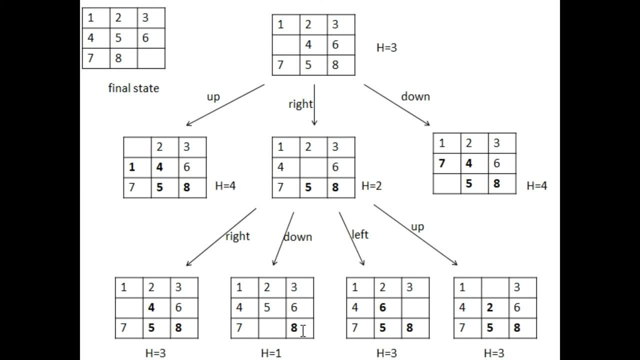 heuristic value is one, because only one tile uh is not at their actual location as required in whole state. so in the same way, the heuristic value for this uh, this state, is three and for this state is three, so just many can get the info bold. for example, two is not at at uh, the at the actual location as required. 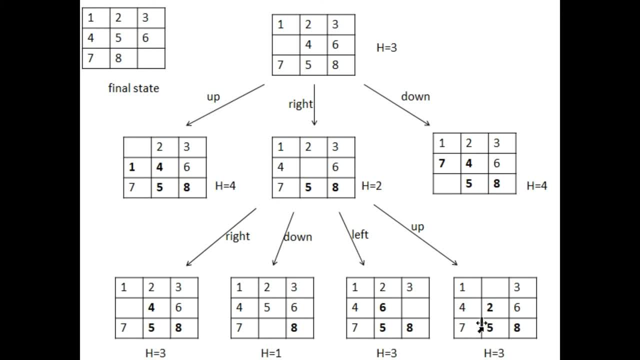 state. in the same way, five and eight, all of these are not at their actual locations as required in our whole state. so the heuristic value up. i will select one node, uh to move, uh to visit the next state. so my case for wizard. then i will pick the, that node which have lowest value of heuristic. so because that node will claim: 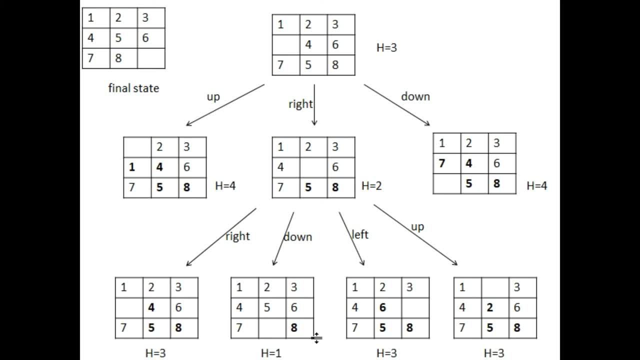 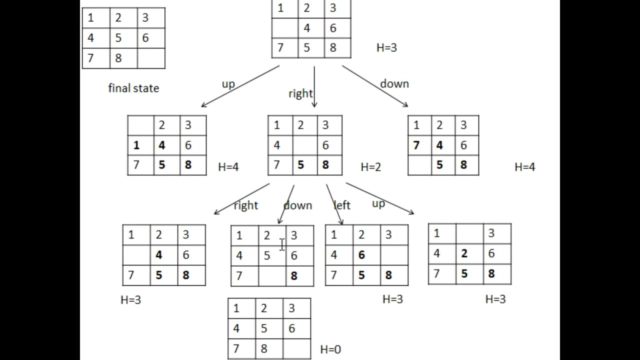 okay, so just look at these four nodes. so i will pick this node. so, um at this state. so just look at the next slide. um is, uh, I will apply the action left. Uhh, so salah. So just look at this problem. That, uh, the this state. so the which is: 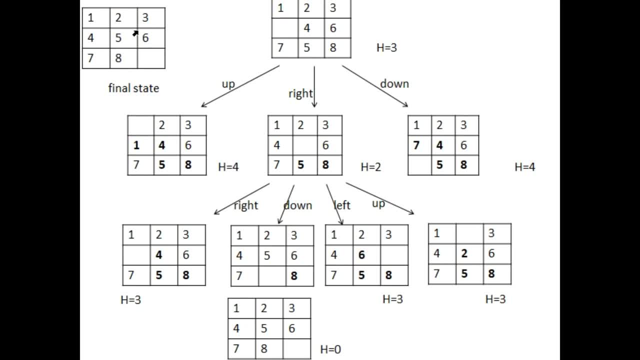 uh, equivalent to our final state. So the path is: uh, Let's first apply the right action on it, then we will apply the down action, and then we will apply the left action, so so then we can achieve the our goal state to reach our. this is our path from. 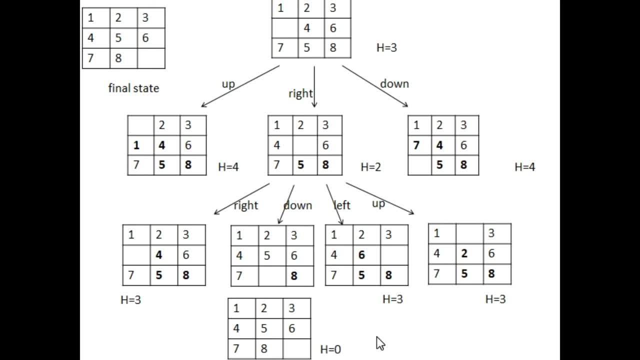 initial state to goal state. so this is how you can calculate your heuristic values: by calculating your initial state of any problem. you can make any function of heuristic value by deciding how to calculate the function value and that function we should have. that, if admissible heuristic returns us. 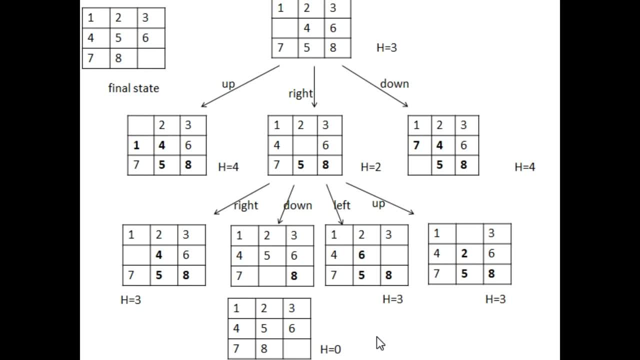 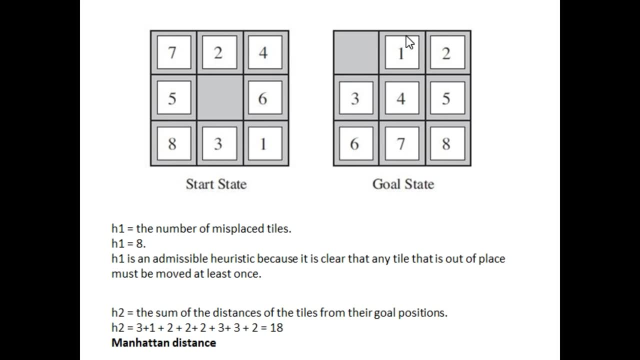 then you can reach the goal state. so in this video lecture we solved this eight puzzle problem by using the heuristic values. basically, the purpose of this lecture is: how can we use heuristic function, how can we generate heuristic values function. so i will. i have generated these two heuristic functions: heuristic values, heuristic.